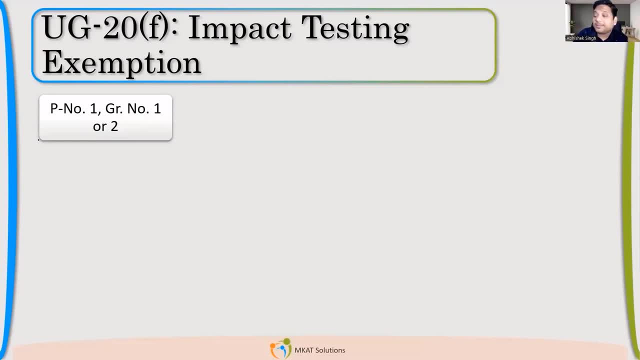 group number one and one or two. So it is basically for p number one material. So there are multiple requirements, Like if I have thickness less than 13 mm And if my material is falling into curve a. Now, what is curve? 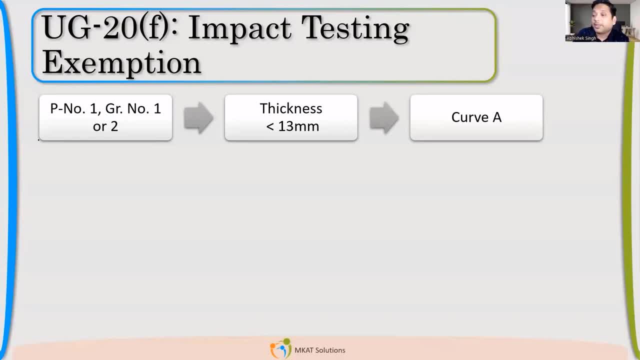 A. what is curve B? I'll you know. if somebody is not aware of that, we'll talk about that also a little bit. but you know, just to remember they are, all the materials falls into different category and also based on whether it they are normalized, not normalized, okay, so what? 20F talks about that. 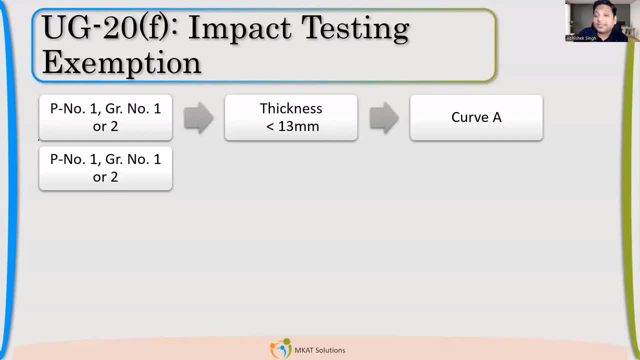 if I have a P number 1 material, my thickness is less than 13 mm and the material is in curve a, in that case I am exempted from impact testing. remember, there are additional requirements which need to be met. okay, so not only this is correct. second, if my thickness is less than 20, 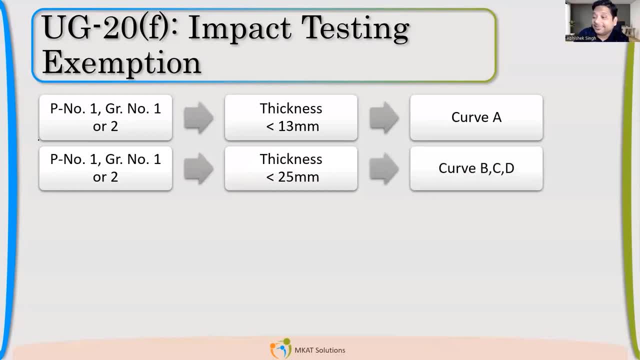 25 and my material in curve b, c, d. so for b, c and d your exemption is extended. okay, they are supposed to be better material, right? that what it seems like, because for those material code is allowing up to 25 mm, I don't have to do impact testing. okay, but now what are the condition under which? 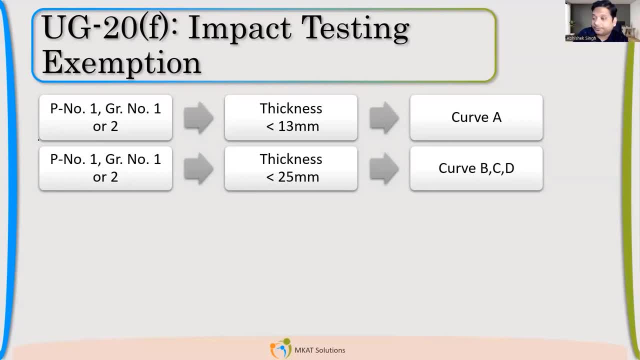 this, these exemptions are allowed. what are those conditions? your vessel should be hydrostatically tested, so that is generally the case. we always do hydrostatic test, so that will be very easily met. second is very important: your design temperature should be between 345 to minus 29 degree Celsius. than only I can apply this if my 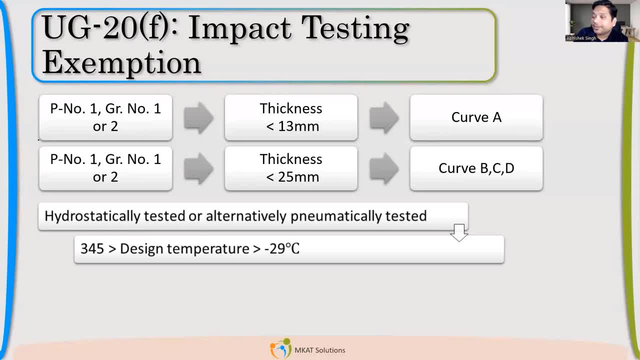 let us say MDMT is given as minus 32, that minimum design temperature from service for minus 29. I cannot take below minus 29. I cannot take that exemption for minus 32. minus 35, it's not permitted, okay, well, this exemption is only allowed.